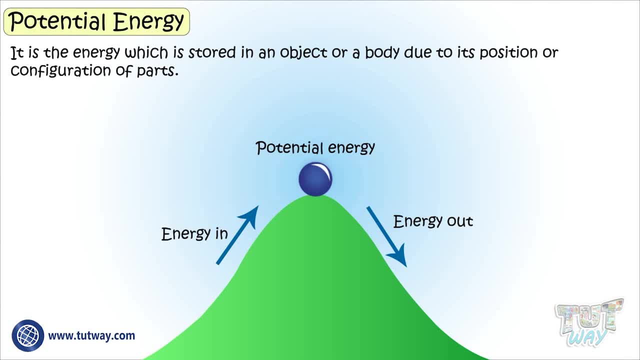 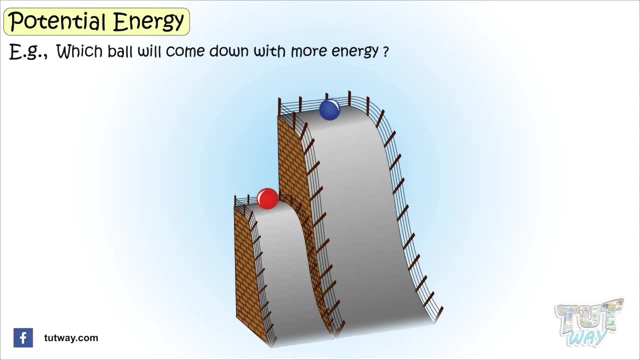 Let's understand it with the help of examples. Which ball will come down with more energy, Blue ball or red ball? Blue ball will come down with more energy, because blue ball had more energy due to more height. But which energy is it? It is potential energy. 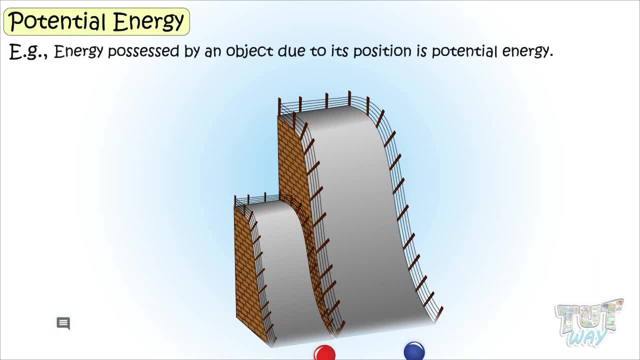 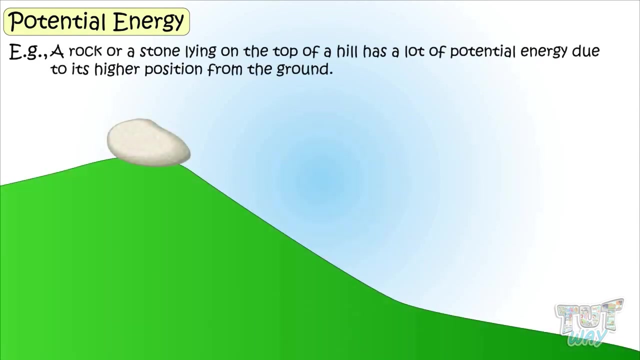 Energy possessed by an object due to its position is potential energy. The higher the position of an object, the more the potential energy. Let's look at another example. A rock or stone lying on the top of a hill has potential energy. Due to its height, it has potential energy. 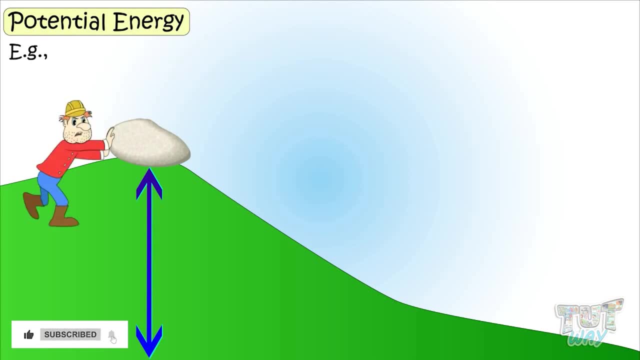 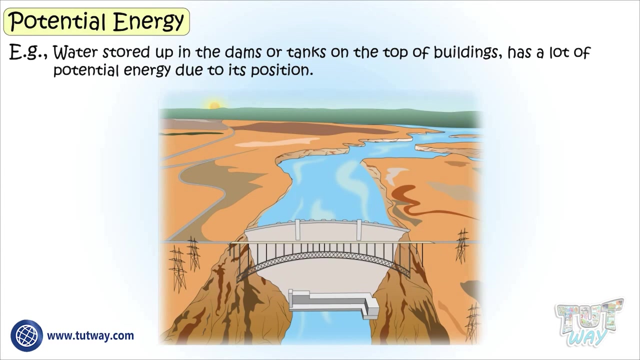 Energy is necessarily there to fill due to its position: higher position from the ground. when this stone is pushed off the hill, it falls down to the ground due to potential energy. Water stored up in the dams or tanks on the top of the buildings have a lot of potential. 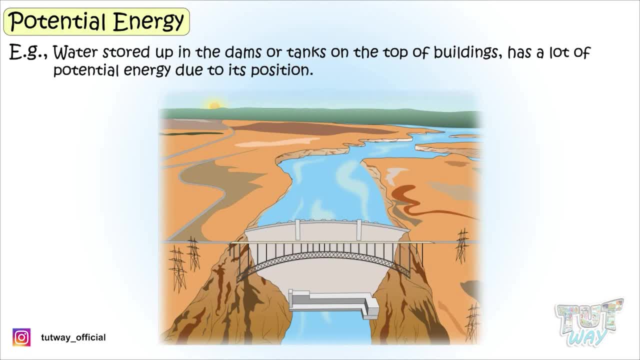 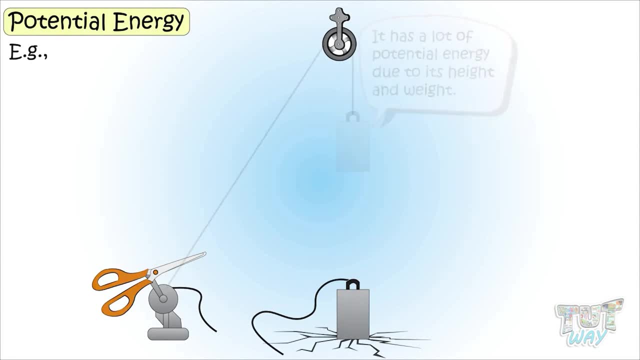 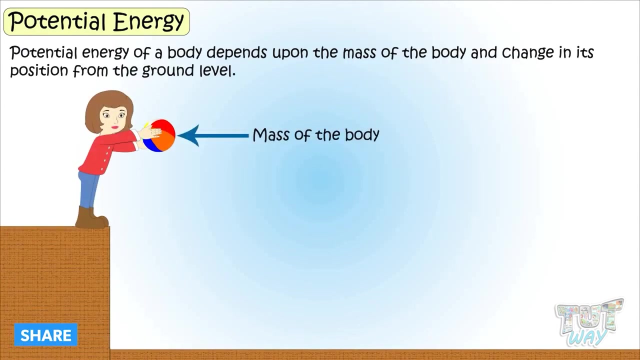 energy due to height. Here is one more example: if we cut the rope, the weight will come down with great energy because it has a lot of potential energy due to its position, that is, its height. but weight too, Potential energy of a body depends upon the mass of the body as well as its position. 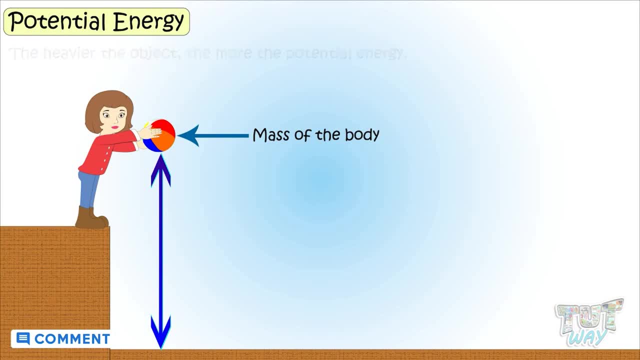 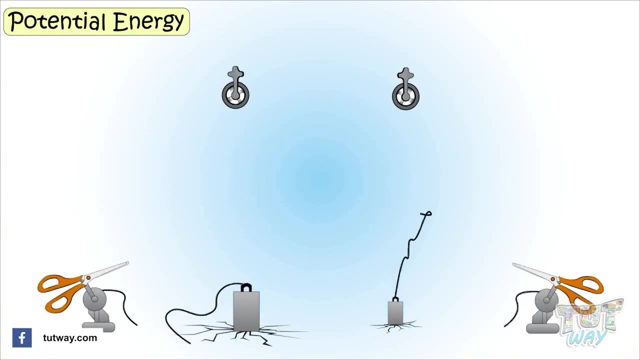 from the ground level. The heavier the object, the more the potential energy. The higher the object, the more the potential energy. Take two different weights now. throw each one by one. Which weight had more energy? Yes, this one, as this has more weight. 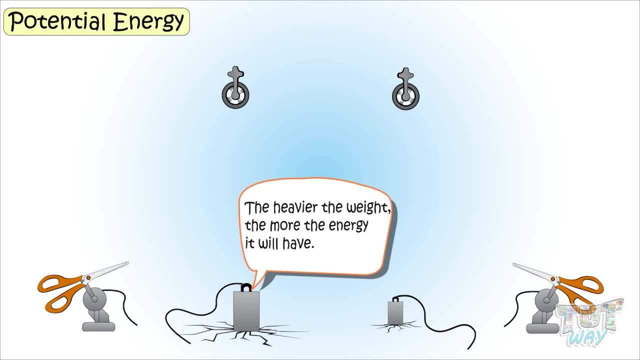 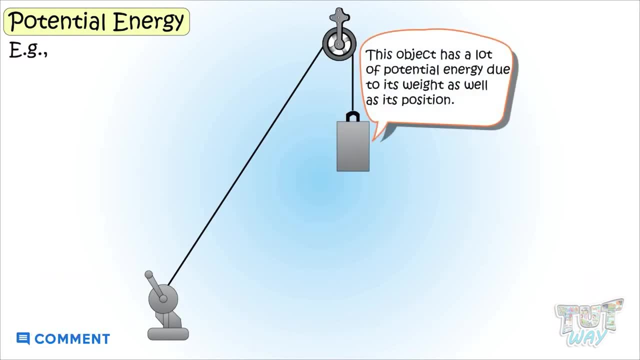 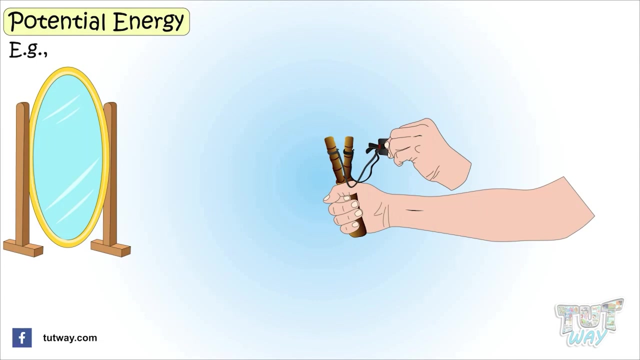 The heavier the weight, more the energy it will have. Now let's take another example. this weight has a lot of potential energy due to its weight as well as its position. It's a catapult, And when the rubber of the catapult is stretched, it stores a lot of potential energy. 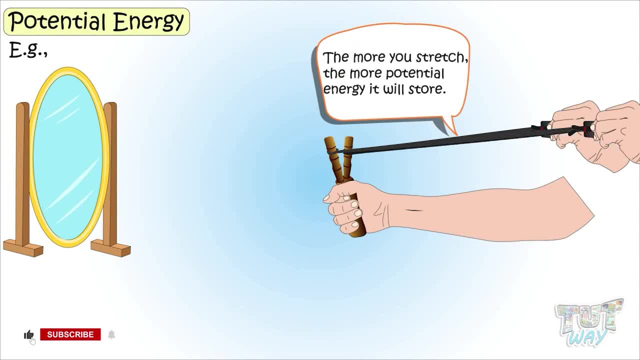 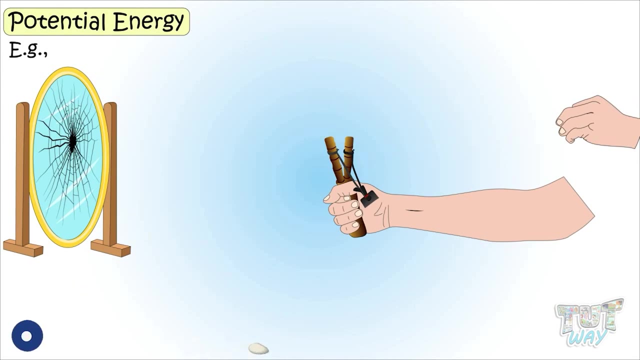 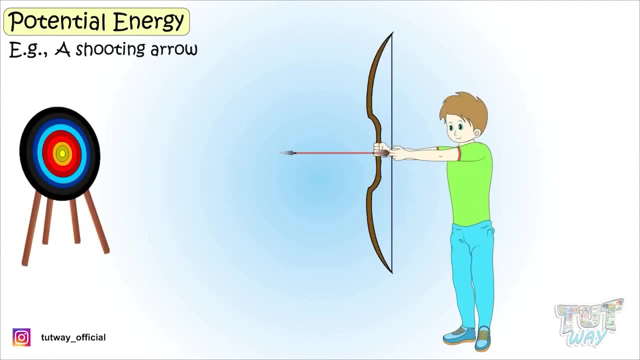 And it's because of its stretched position. The more you stretch, the more potential energy it will store this potential energy stored in it. when you release the stretch rubber, it throws the stone with a great energy. Bow and arrow- Bow and arrow- also works on the same principle. 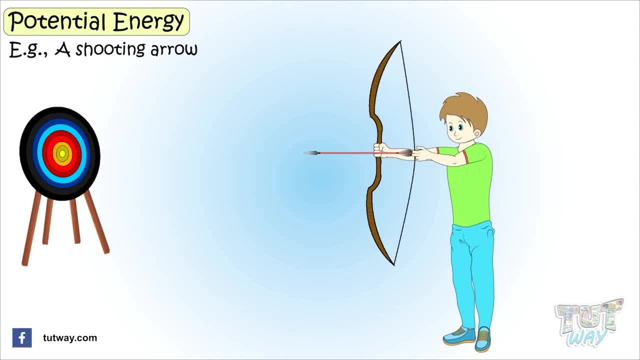 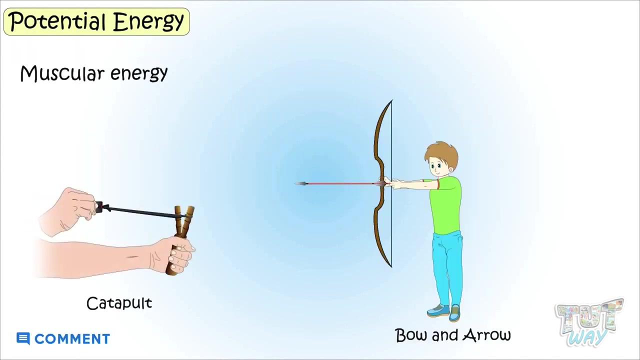 The arrow is held on the stretch string of the bow and due to this stretch position, a lot of potential energy is there. The more it is stretched, the more potential energy it will store and with more force the arrow will go ahead. In both these examples it is first a muscular energy. 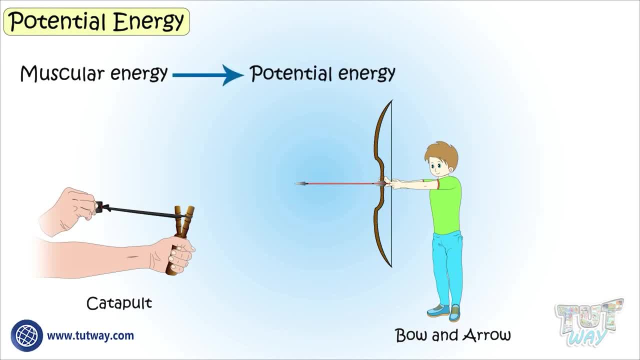 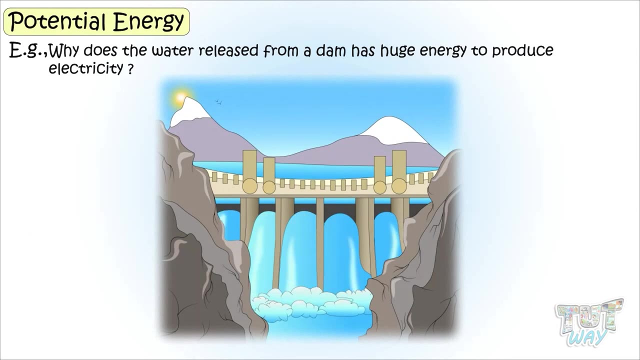 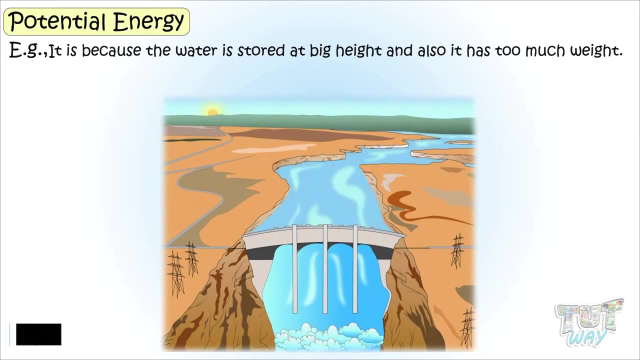 which is being converted to the potential energy, and then the potential energy is being converted to the kinetic energy. Now let's see another example. Why does the water released from a dam has huge energy to produce electricity? It is because the water is stored at big heights and also the quantity of water has too much weight. 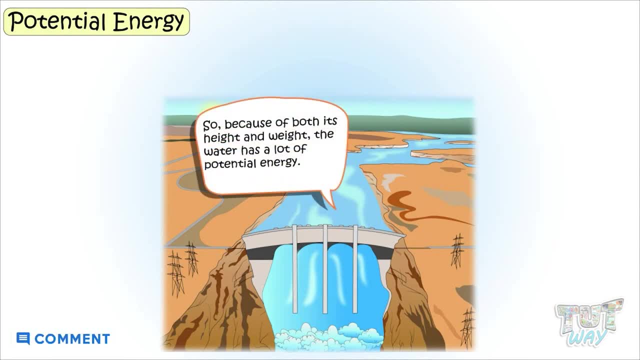 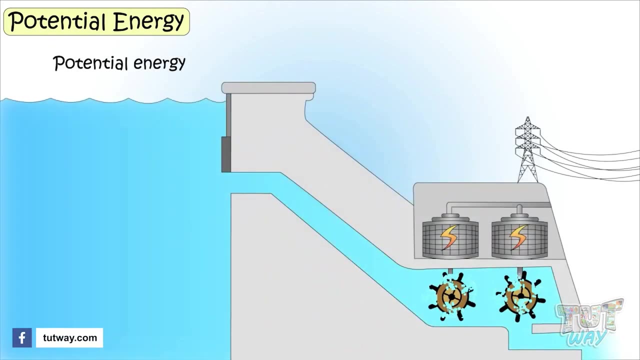 So, because of both height and weight, when the water from the dam is released from a great height, it has enormous potential energy. This potential energy of the water is converted to kinetic energy and gives it a great speed, And this kinetic energy is used to move the turbines, which in turn powers the generators that